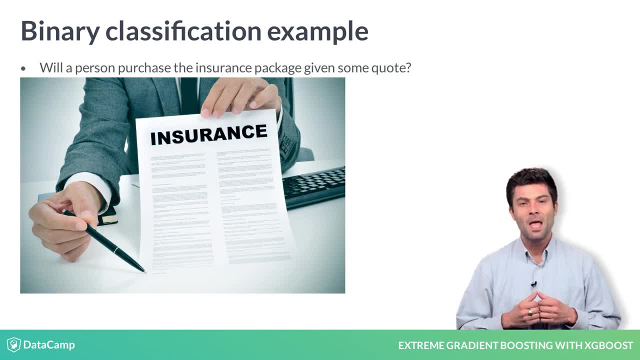 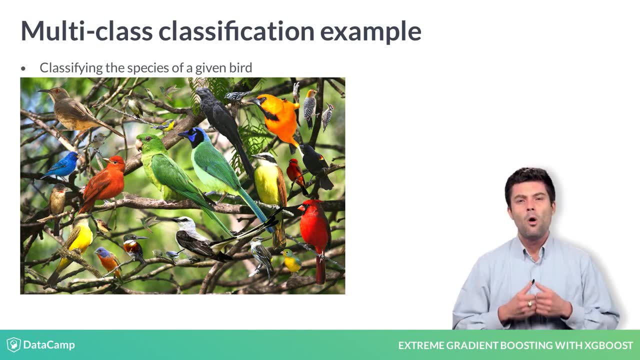 package given some quote is a binary supervised learning problem, and predicting whether picture contains one of several species of birds is a multi-class supervised learning problem. When dealing with binary supervised learning problems, the AUC or area under the receiver operating system should be used for the identification of the image or the. 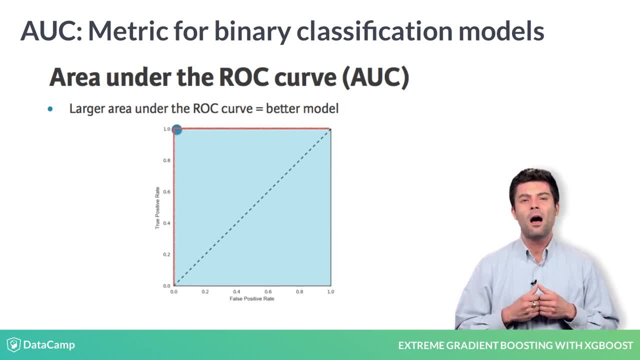 operating characteristic curve is the most versatile and common evaluation metric used to judge the quality of a binary classification model. It's simply the probability that a randomly chosen positive data point will have a higher rank than a randomly chosen negative data point. for your learning problem. So. 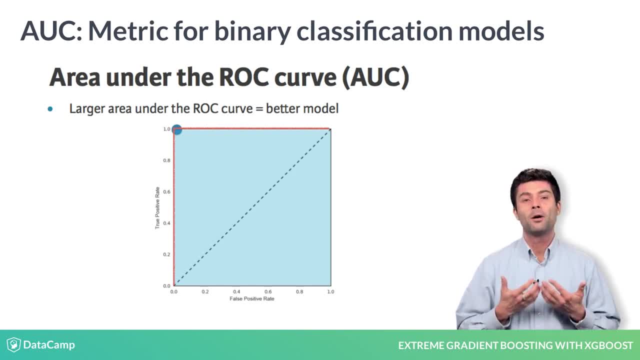 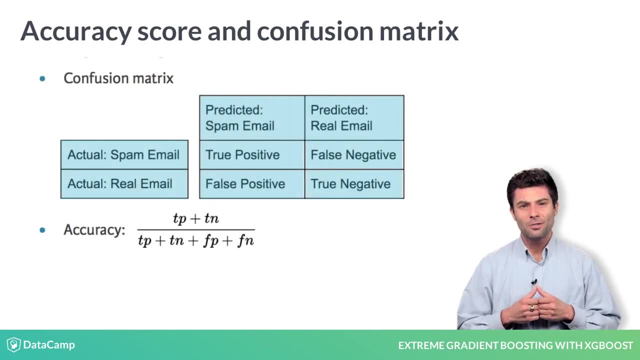 a higher AUC means a more sensitive, better performing model. When dealing with multi-class classification problems, it is common to use the accuracy score- higher is better- and to look at the overall confusion matrix to evaluate the quality of a model. Some common algorithms for classification problems: 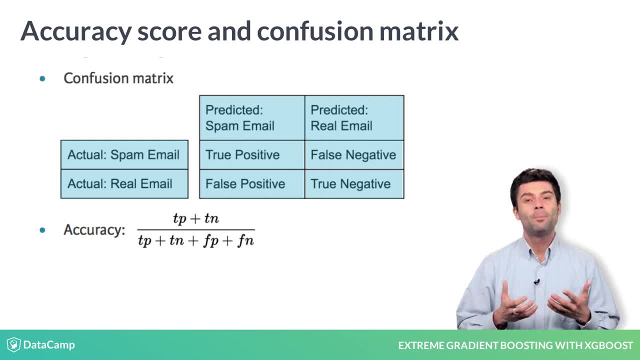 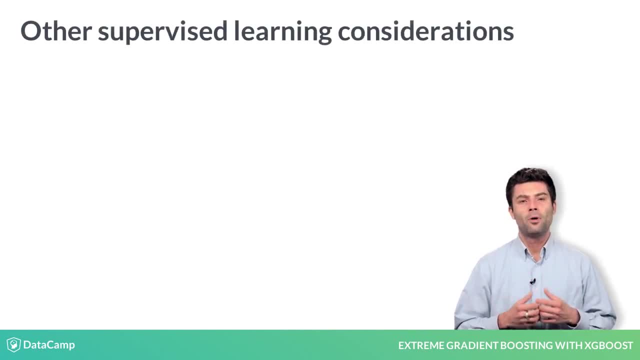 include logistic regression and decision trees. If you want a deeper review, check out DataCamp's introductory course on supervised learning. All supervised learning problems, including classification problems, require that the data is structured as a table of feature vectors, where the features themselves 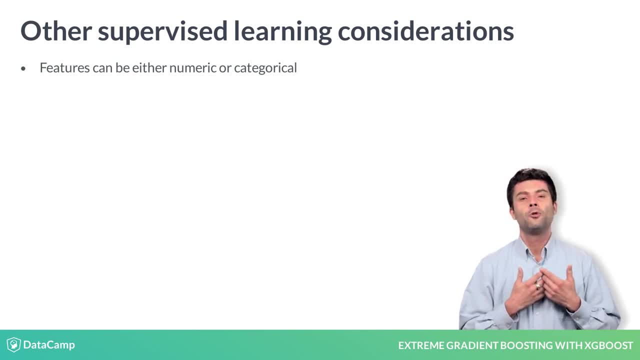 also called attributes, are defined. In this case, the attributes, or predictors, are either numeric or categorical. Furthermore, it's usually the case that numeric features are scaled to aid in either feature interpretation or to ensure that the model can be trained properly. For example, numerical feature scaling is essential to ensure properly. 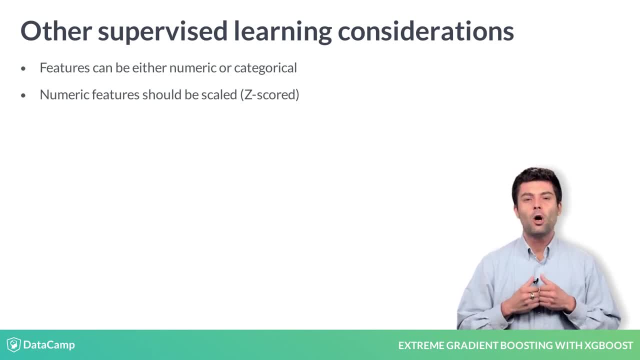 trained support vector machine models. Categorical features are also almost always encoded before applying supervised learning algorithms, most commonly using one-hot encoding. Finally, other kinds of supervised learning problems exist, so I'll mention them here briefly. Ranking problems involve predicting and ordering on a set. 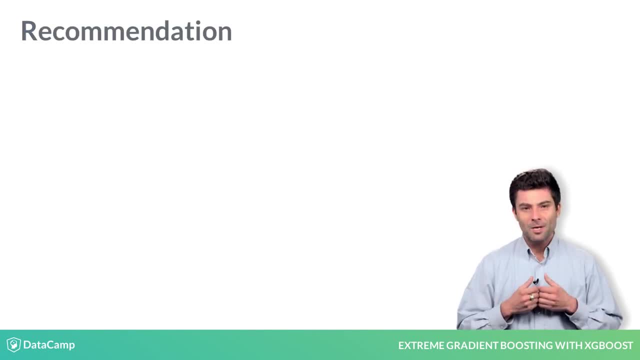 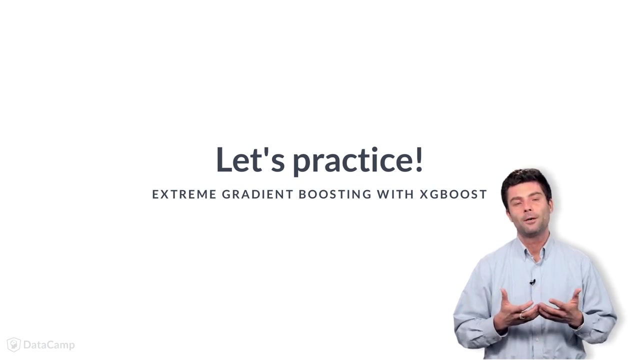